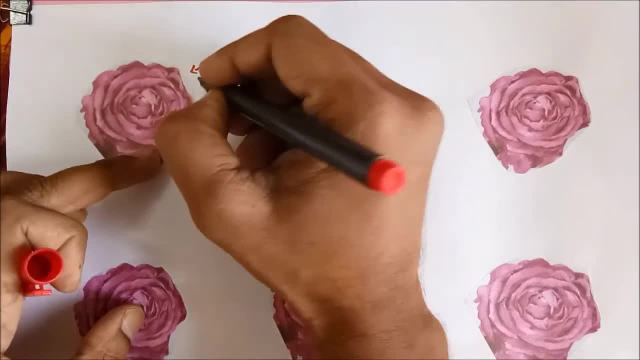 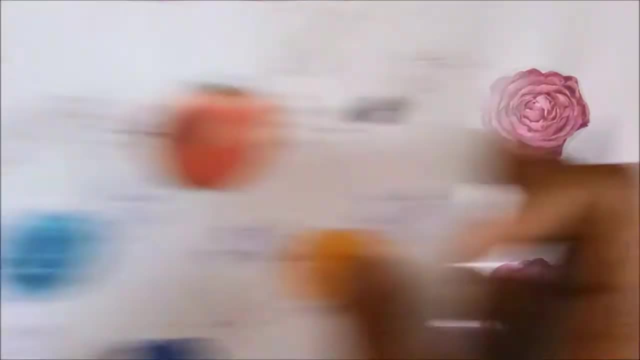 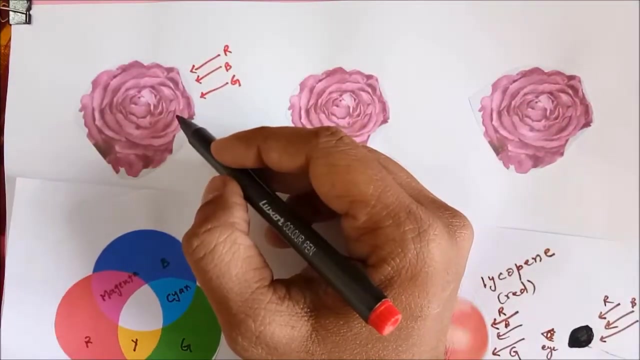 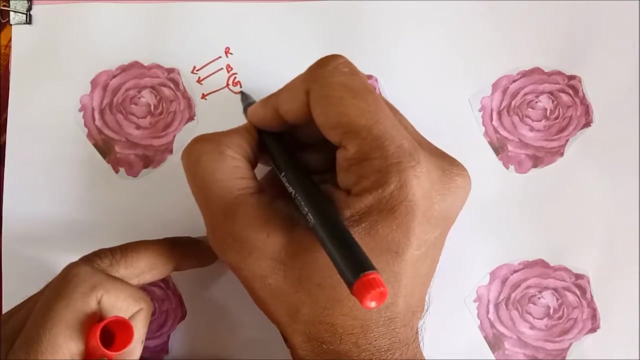 So let us impart white light on it. White light is made up of red, blue and green. Now, magenta is made up of red and blue. So the pigments in this flower are going to absorb its complementary color, that is green. So the green light is going to get absorbed. red and blue are not going to. 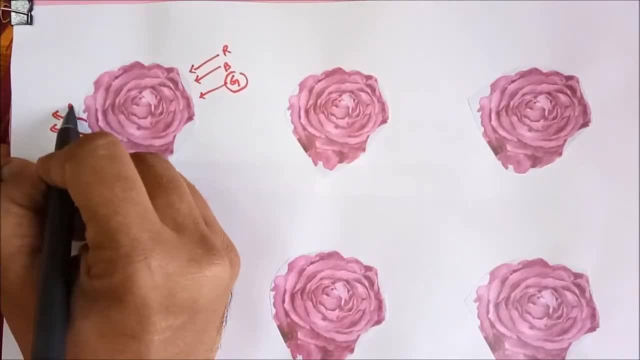 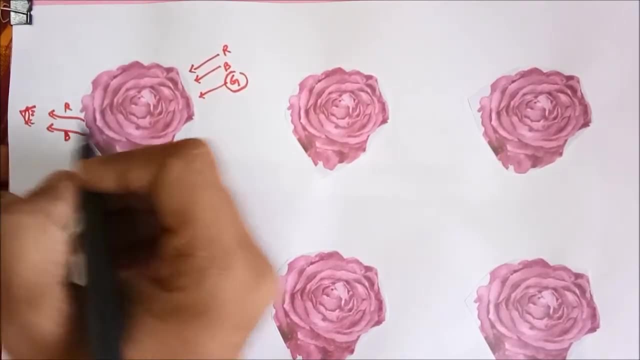 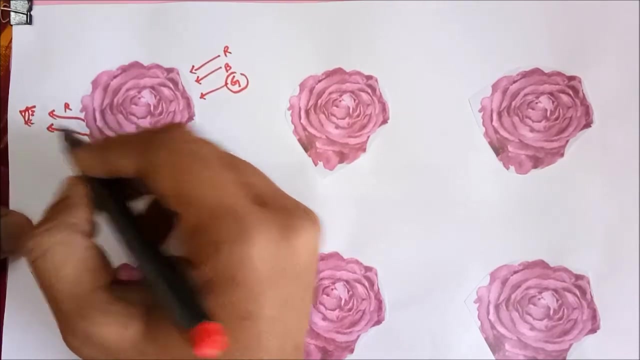 get absorbed. So red and blue are going to be present in the reflected light and they mix together to form magenta color. So in white light green gets absorbed, red and blue combine together to form magenta finally reaching our eye. So we see magenta color of this rose in white light. 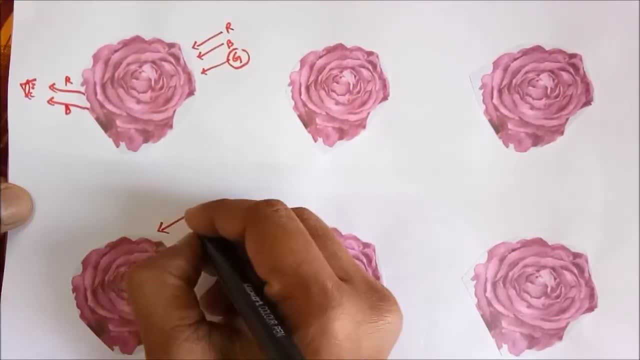 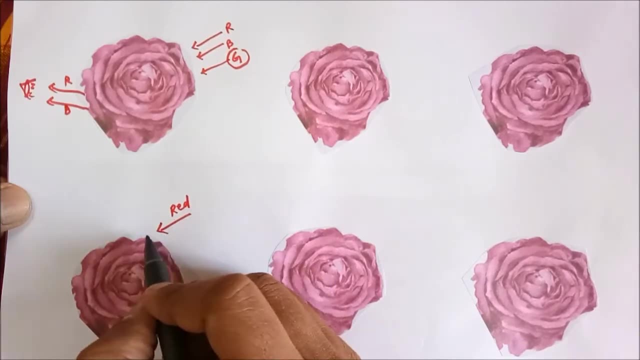 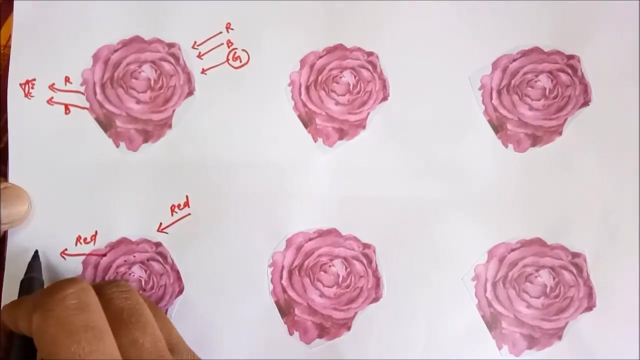 Okay, let us impart some red color light on it. We know that it only absorbs green color, So the red light falls on it and these pigments are not going to absorb this red light. So the red light is present in the reflected light and finally we perceive the color. 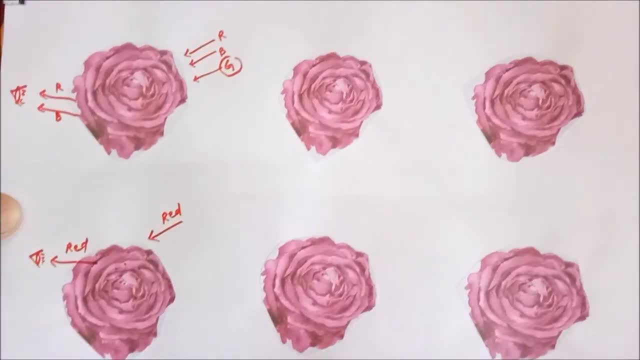 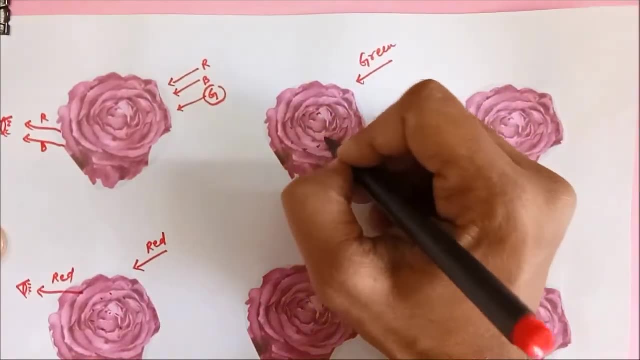 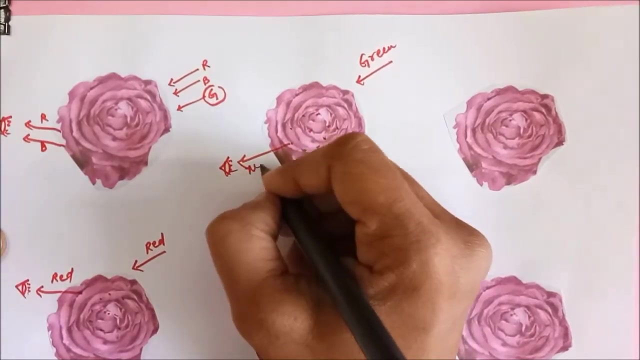 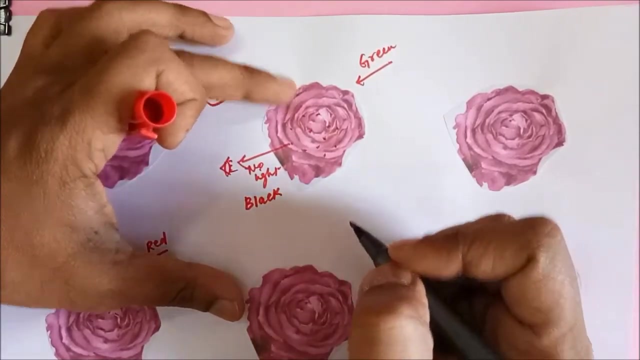 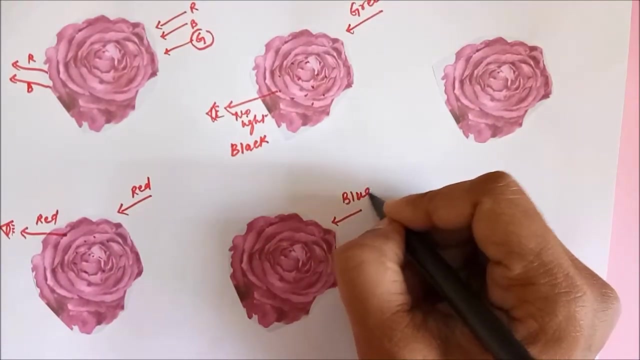 of this rose as red in red light. Let us take green color. This green color will be totally absorbed by the pigments inside, So nothing reaches our eye. and when no light reaches our eye, we see this as black. right, Okay, let us impart blue color on it. Blue also does not get absorbed. 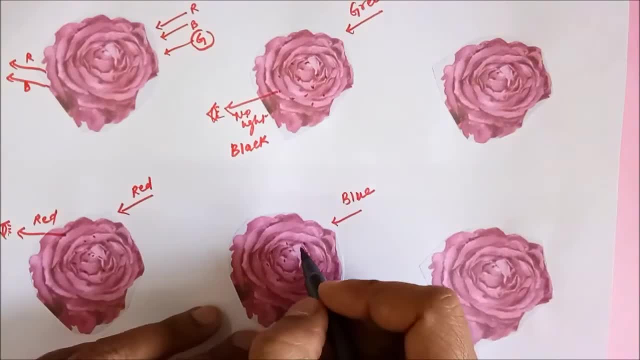 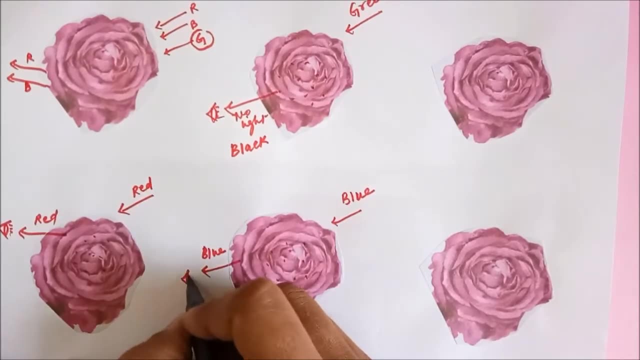 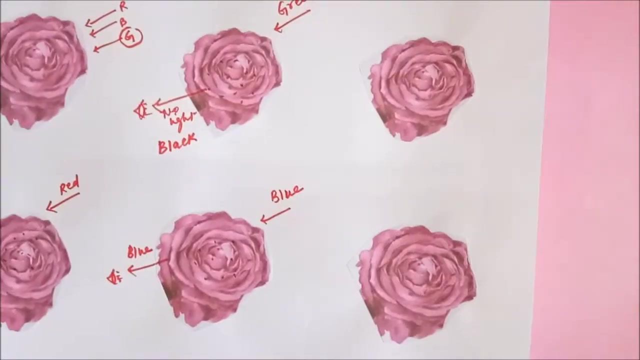 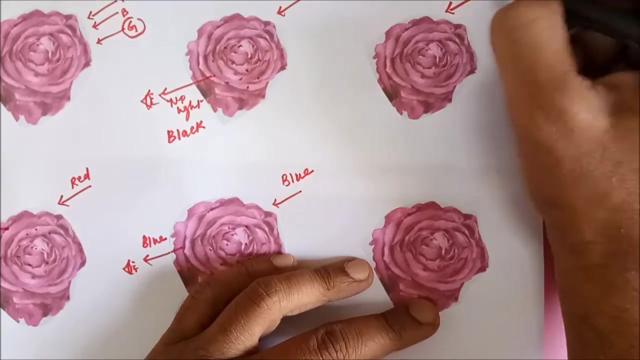 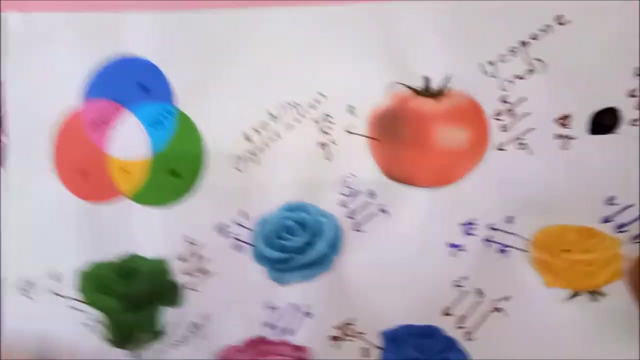 Pigments are only capable of absorbing the green light, So blue gets reflected, totally, reaches our eye. So we perceive this rose as blue in blue light. And if we use cyan color or if we use cyan light on it, cyan light is made up of blue and green, So we can also write like this: that blue